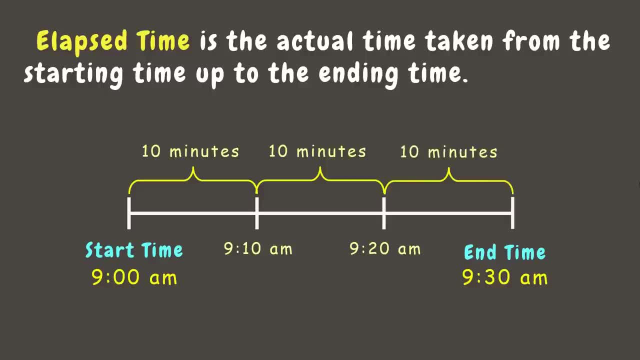 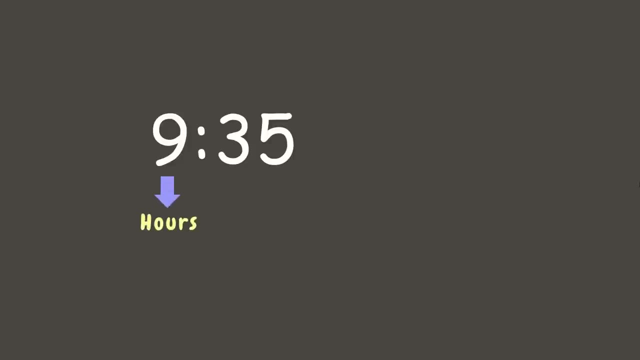 it will be 9.30 am. If we combine these times taken, we have 30 minutes as the elapsed time. Now let's have a quick review about time In 9.35,. 9 represents the number of hours. 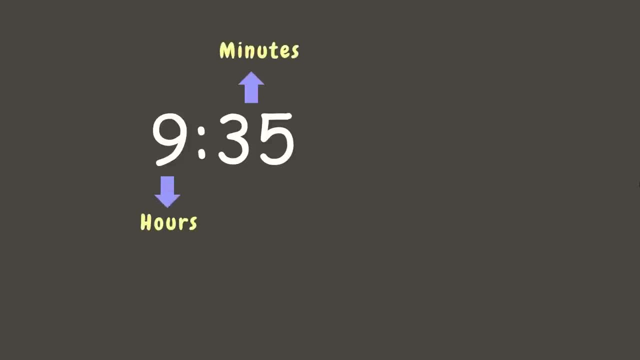 while 35 is the number of minutes. If we add another one here, 19 represents the number of seconds, while am and pm refers to the meridiem. Am stands for ante meridiem, which means from midnight until morning before noon. 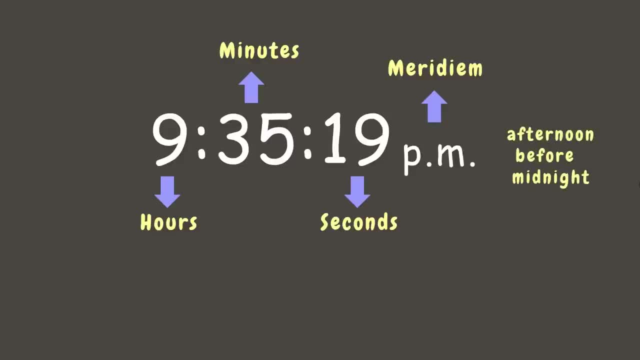 while pm stands for post meridiem, which means afternoon until before midnight. Another thing that you should know is that one hour is equals to 60 minutes and one minute is equal to 60 seconds. We will use this later on. 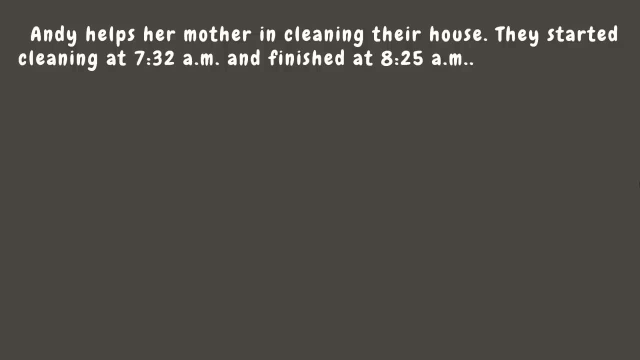 Now going back to our problem. we have two ways of finding elapsed time. First one is by using a number line. Let's make a number line starting from 7.30 am, skipping every 5 minutes up to 8.25 am. 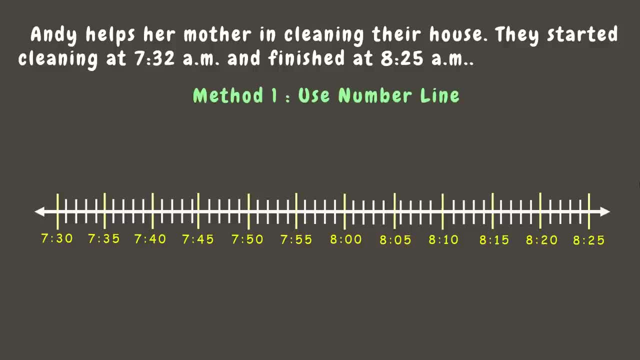 There you go In the number line. here is the start time, which is 7.32 am, while 8.25 is the end time. Now let's count the number of minutes from start time up to the end time. 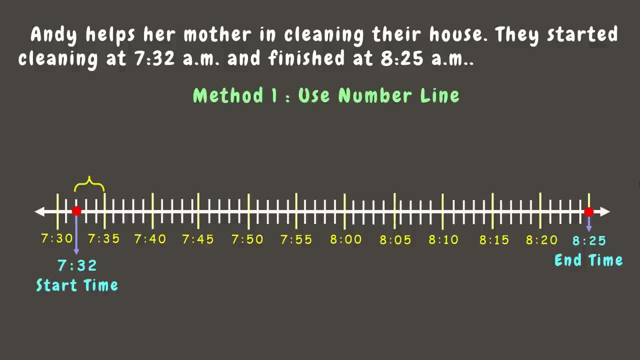 Starting from 7.32 to 7.35, we have 3 minutes. From 7.35 to 7.40, we have 5 minutes. Same with 7.40 to 7.45, which is also 5 minutes. 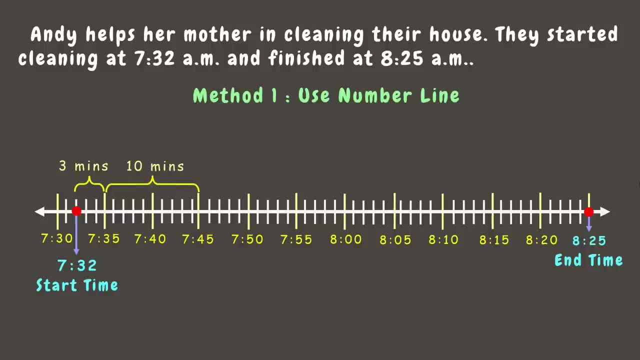 If we combine this, they are 10 minutes. Same from: 7.45 to 7.55 is 10 minutes. 7.55 to 8.05 is 10 minutes. 8.05 to 8.15 is also 10 minutes. 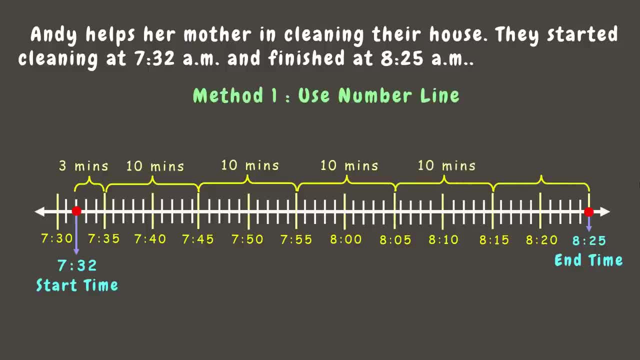 And lastly, 8.15 to 8.25, which is our end time- is another 10 minutes. If we combine these times taken, we have exactly 53 minutes, which is our total elapsed time. Now let's see if our end time is 10 minutes. 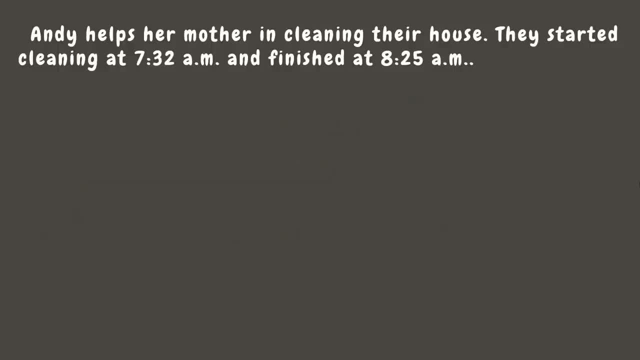 Our answer is the same using our second method, which is subtraction. Remember this example is only applicable at start time and end time are either both am or both pm. Here, in our problem, the start and end time are both am. 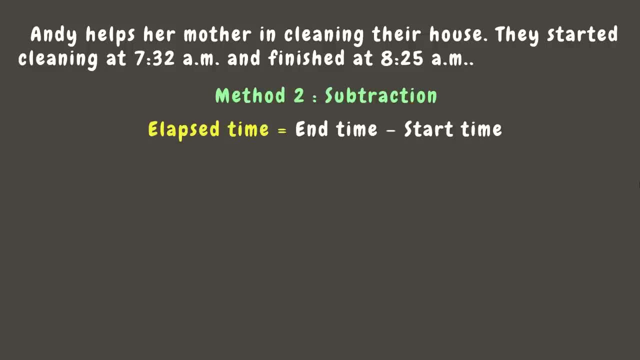 Now to solve for the elapsed time, simply subtract the start time from the end time. Here, the end time is 8.25.. 8.25 am minus the start time, which is 7.32 am. 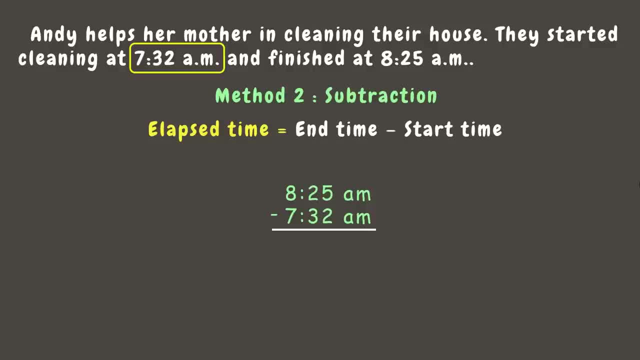 Now let us subtract from right to left, starting from minutes. Here we can see that 25 is smaller than 32, which means we cannot subtract this right away. We need to borrow first from hours. Now let's borrow one hour from 8.. 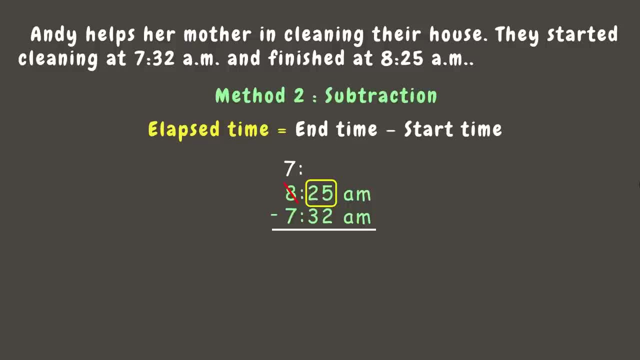 Now 8 becomes 7.. Then let's add one hour that we borrowed to 25 minutes. But first let's convert one hour to minutes. We know that one hour is equal to 60 minutes. Therefore, let's add 60 minutes to 25, which is 85 minutes. 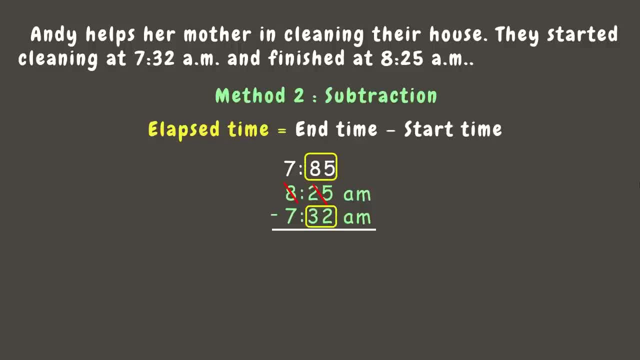 Now let's subtract: 85 minus 32 is 53, while 7 minus 7 is 0. Therefore, our answer is 53 minutes, Which means This means they cleaned the house for exactly 53 minutes. Great job. 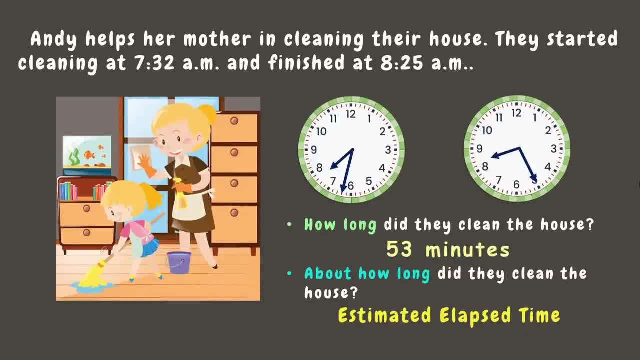 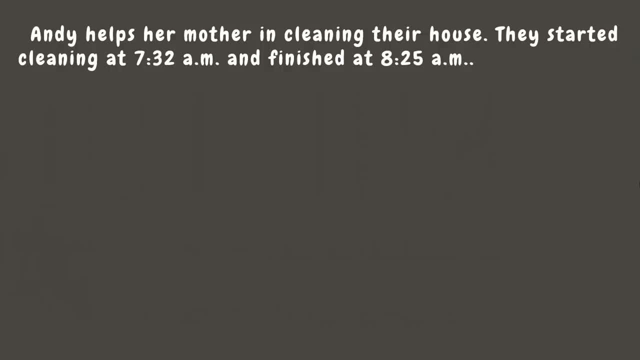 We already found the elapsed time, which is 53 minutes. Next let's find out its estimated elapsed time. Let's use the subtraction method To find estimated elapsed time. subtract estimated start time from estimated end time. First let's write down the actual times. 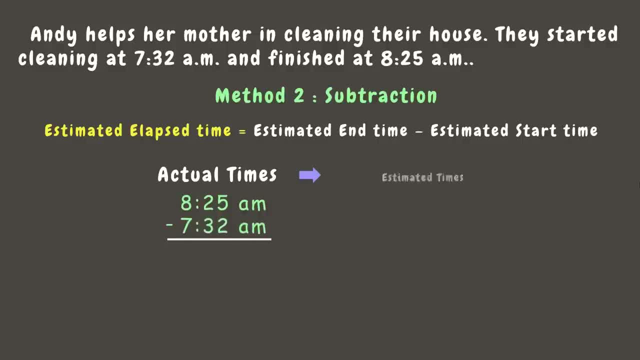 There you go. We can get the estimated times by rounding off the minutes of each time. The rounded time for 8.25 is 8.30 AM, while 7.32 will be 7.30.. Now let's subtract. 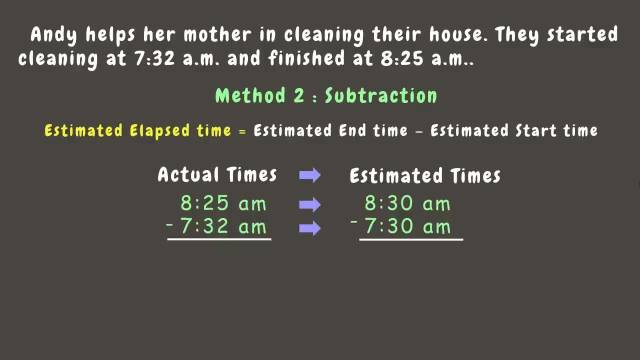 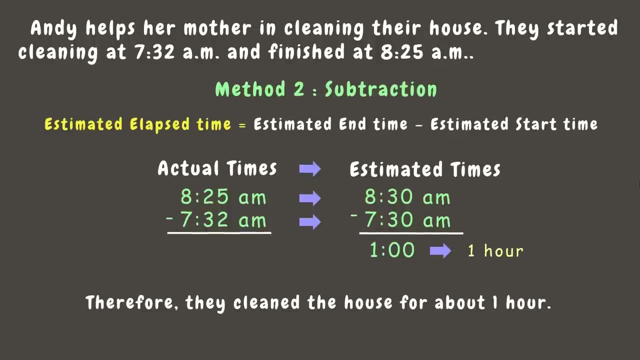 30 minus 30 is 0. And 8 minus 7 is 1.. Therefore, our answer is 1 hour. Therefore, they cleaned the house for about 1 hour. Good job, We now got the estimated elapsed time, which is about 1 hour. 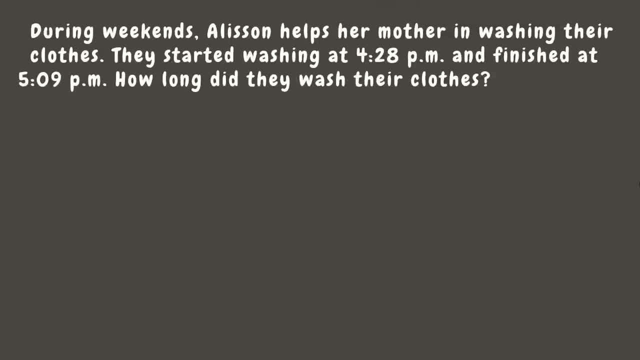 Now let's have more examples. During weekends, Allison helps her mother in washing their clothes. They started washing at 4.28 PM and finished at 5.09 PM Again. to find the elapsed time simply subtract time from the end time. 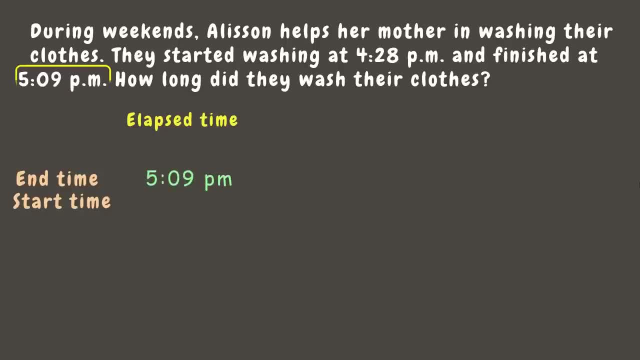 End time here is 5.09 PM minus the start time, which is 4.28 PM, Since 9 is smaller than 28,. it means that we need to borrow 1 hour from 5.. Now 5 becomes 4.. 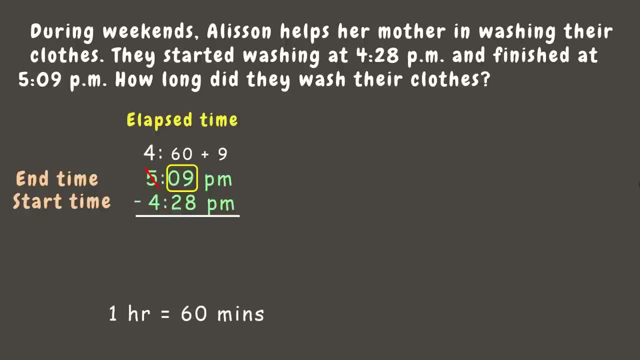 Now let's add 1 hour, which is 60 minutes, to 9,, and that is 69.. Now let us subtract: 69 minus 28 is 41,, while 4 minus 4 is 0.. Now we got 41 minutes. 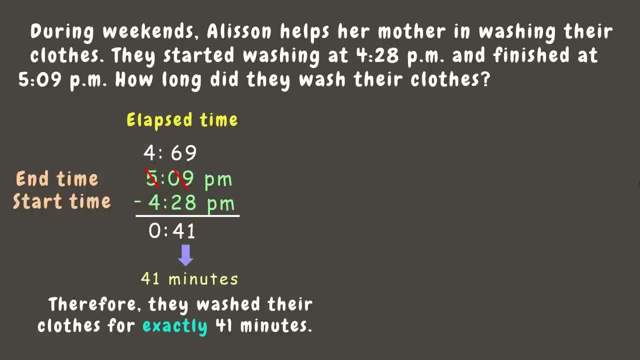 Therefore, they washed their clothes for exactly 41 minutes. Now let's try to get its estimated elapsed time. Let's round off 5.09 PM, which is 5.10, while 4.28 is 4.30. 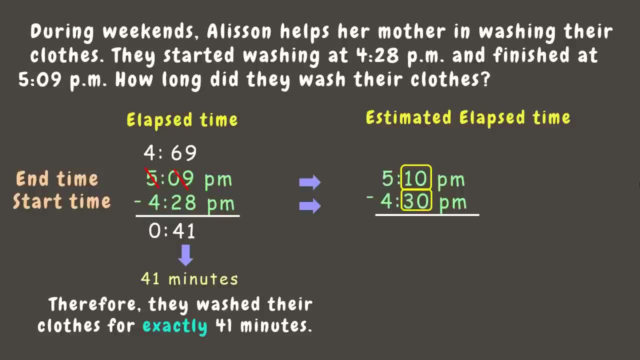 Let's subtract, Since 10 is smaller than 30, it means that we need to borrow 1 hour from 5.. Now 5 becomes 4.. Then let's add 1 hour, which is 60 minutes, to 10, and that is 70.. 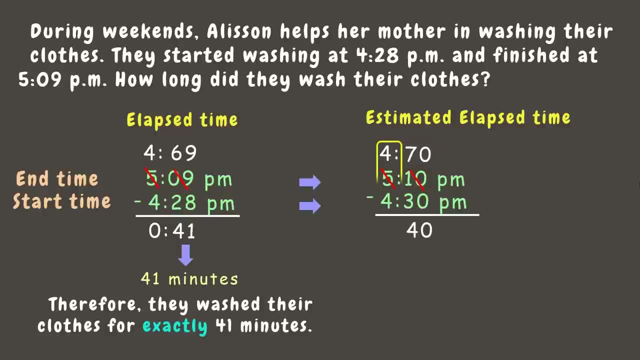 Now, 70 minus 30 is 40, while 4 minus 4 is 0. Therefore, we got 40 minutes. Therefore, they washed their clothes for about 40 minutes. Awesome. Now I'll give you more examples. 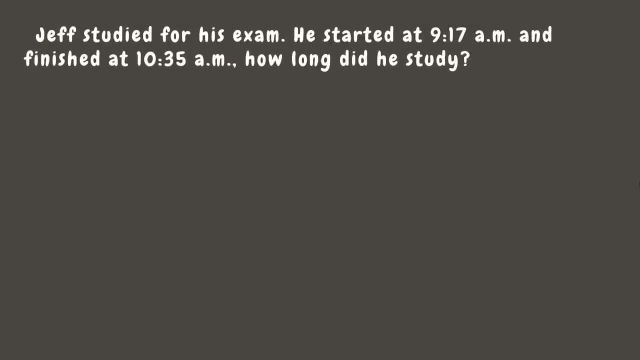 Jeff studied for his exam. He started at 9.17 AM and finished at 10.35 AM. How long did he study? Remember to find the elapsed time, simply subtract start time from the end time. End time here is 10.35 AM, while start time is 9.17 AM. 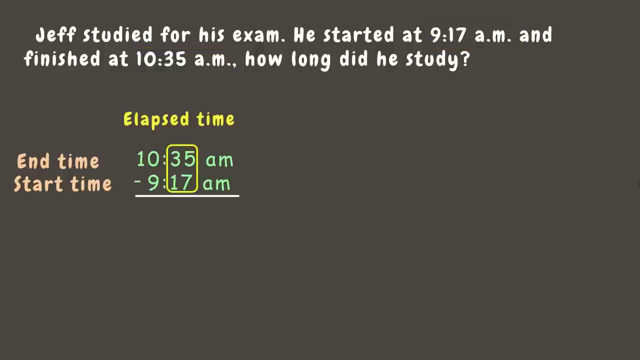 Let us subtract, Since 35 is bigger than 17,. we don't need to borrow from hours anymore. We can subtract this right away: 35 minus 17 is 18, while 10 minus 9 is 1.. We got 1 hour and 18 minutes. 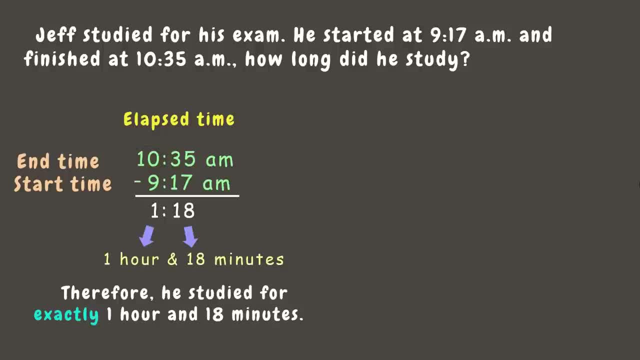 Therefore, he studied for exactly 1 hour and 18 minutes. Now let's try to get his estimated elapsed time. Let's round off 10.35, which is 10.40 AM, While 9.17 is 9.20 AM. 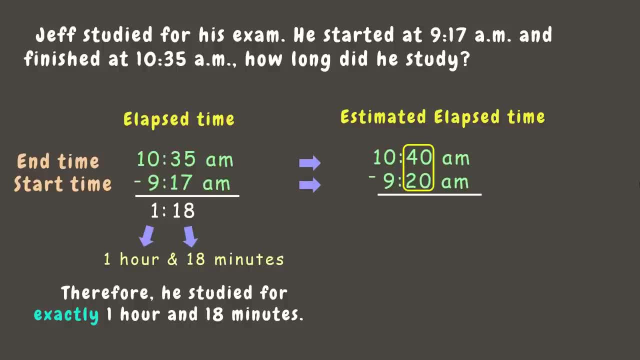 Let us subtract: 40 minus 20 is 20, while 10 minus 9 is 1.. Now we got 1 hour and 20 minutes. Therefore, he studied for about 1 hour and 20 minutes- Great, 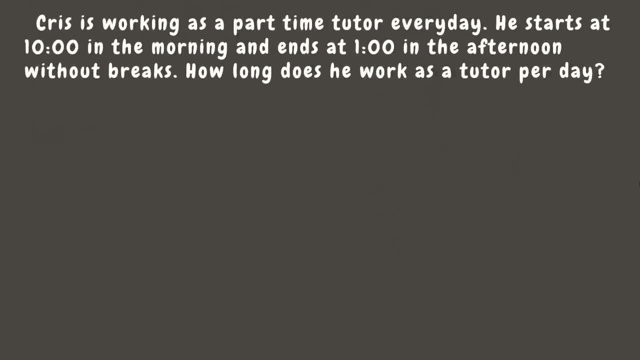 Now let's go to our last example. Chris is working as a part-time tutor every day. He starts at 10 o'clock in the morning and ends at 1 o'clock in the afternoon, without breaks. How long does he work as a tutor per day? 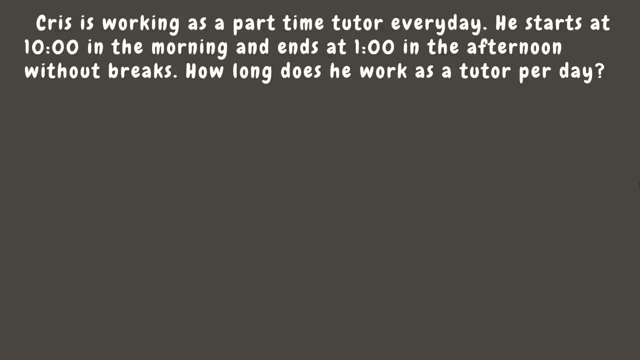 Let's try answering this first using a number line, Starting from the start time, which is 10 in the morning or 10 AM, up to the end time, which is 1 o'clock in the afternoon, which is 1 PM. 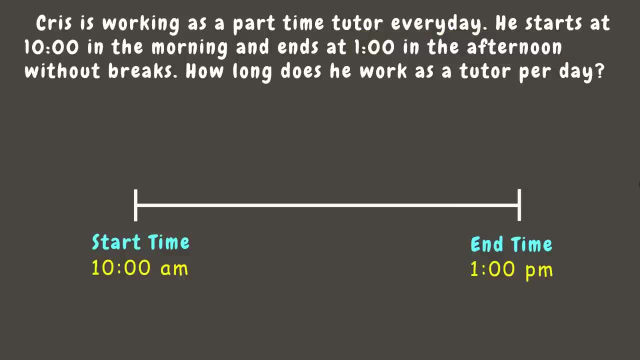 If we try to add 1 hour to 10 AM, which is our start time, the time will be 11 AM. If we add 1 more hour, it will be 12 noon, And if we add another 1 hour, we will reach our end time, which is 1 PM.